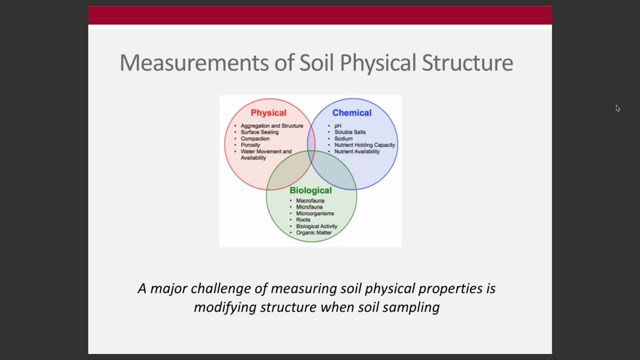 Okay, so focus on soil chemistry for soil testing for many decades, and now we have a resurgence for looking at soil biological activity, looking at physical structure. how are we going to do this? So major challenge of measuring soil physical properties is that we modify soil structure every time we soil sample right. 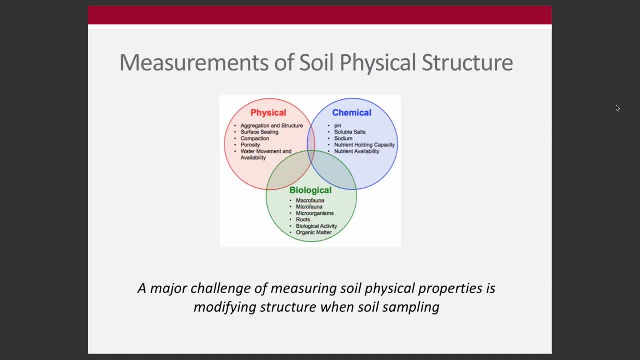 So think about how we take a soil sample or how we actually often analyze soils. The first step is we go out and we take a probe, sink it in the ground, we collect that soil, take it back to lab and one of the first things we do we might push it through a sieve and just to try to homogenize the different cores and mix them together. 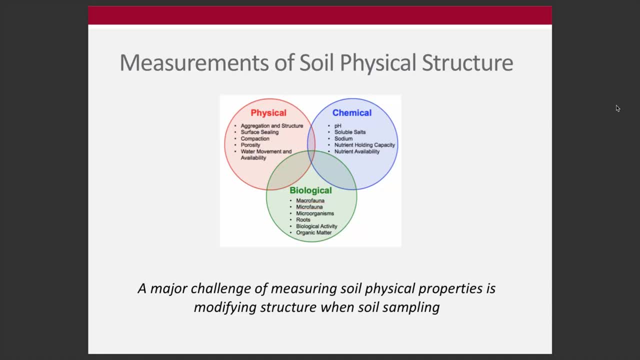 What a commercial lab will do is the first thing they'll do is they'll dry, typically overnight, and then they'll often grind that sample to have it pass through a two millimeter sieve. And so you know, with that grinding, of course, or with that sieving, whatever we do to make it more homogenous, we're absolutely modifying in a very major way that soil structure right. 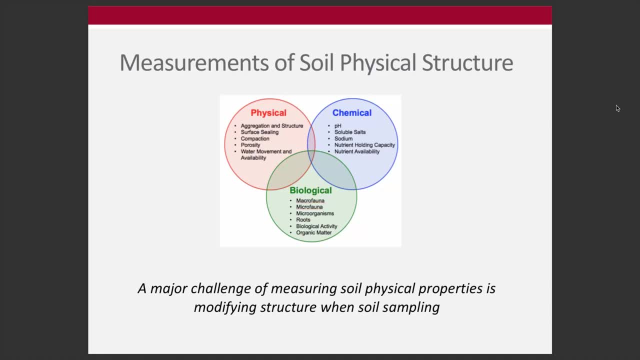 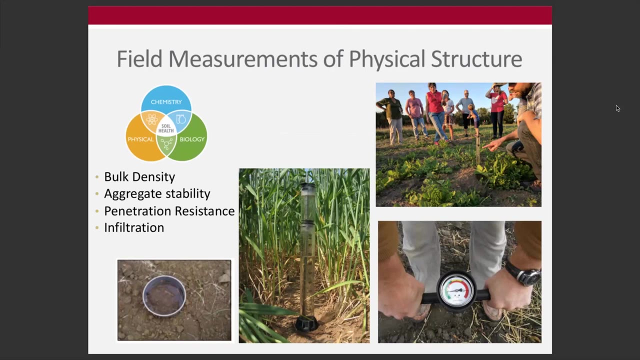 So we either have to measure it on intact cores or we've got to do it in the field. So it's really challenging to do this, to actually measure soil physical structure when we are pulling soil samples. So because of that we often go and think about measuring things in the field. 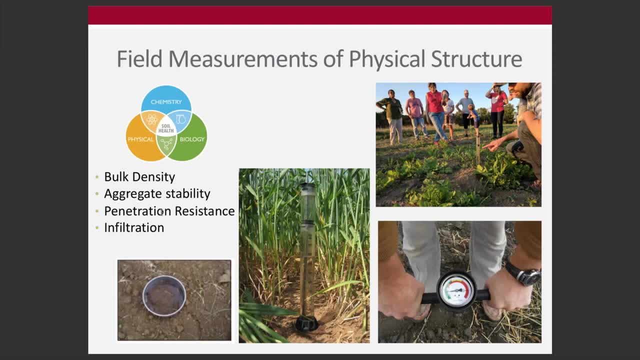 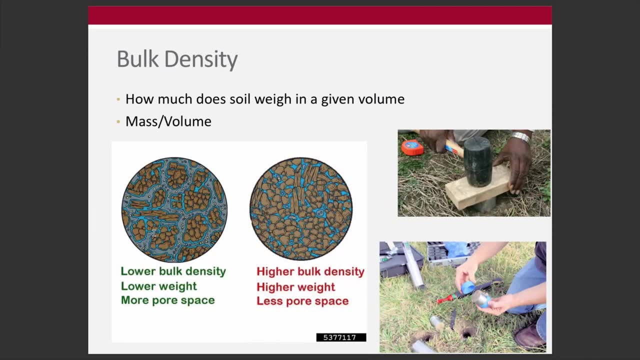 So we can do things like bulk density, aggregate stability, penetration, resistance and infiltration. So these are. I'll just run through each one of these. Bulk density is a you know kind of classic common soil measurement, Been around for a long, long time. 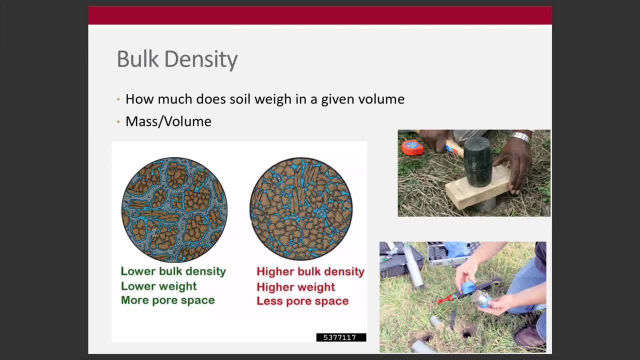 It's this idea of how much does a soil weigh in a given volume. That's really the measurement. What's the mass of soil per unit of volume? And it has to do with porosity and pore space and lower bulk density values equal more pore space and lower weight. 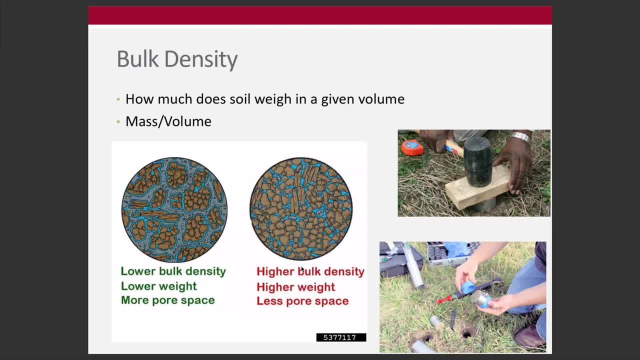 Higher bulk density values equal less pore space and more mineral material per volume. Okay, We typically do this by pounding a core- different ways to do this- but we basically pull a core in to the ground, We pull it out, We shave carefully, shave, you know, excess off and we get a common volume. 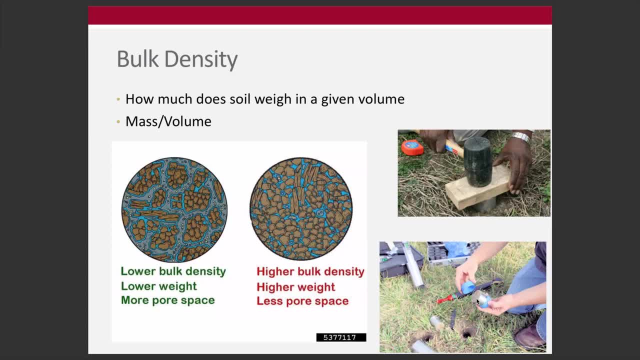 We dry this and we weigh it and you get a mass, And so our cylinder remains fixed. so we know that volume and then we just take the weight. Okay, So it's a common, not particularly easiest measurement to take in the world, because there's some nuance to this. 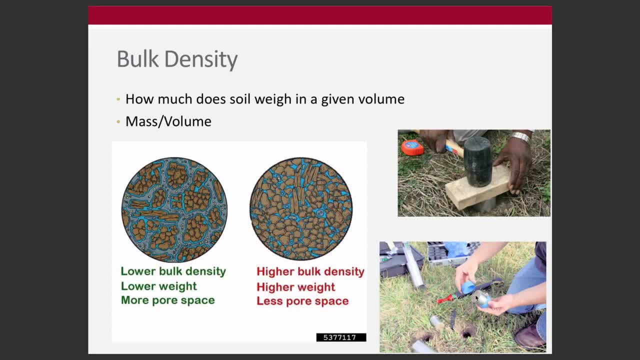 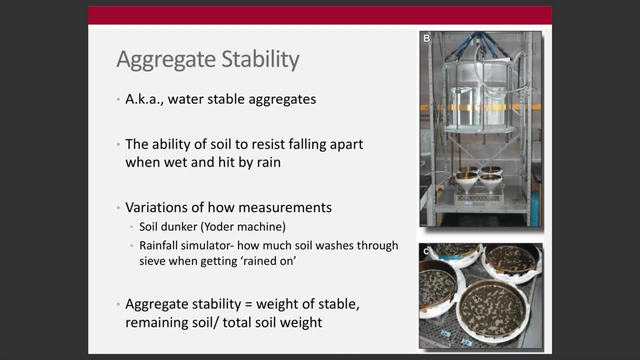 But it's- you know, it's something that's commonly done in soil science- Aggregate stability or water stable aggregates. So this is really the ability of aggregates to resist falling apart when hit by water or rain or wind. The microbial glue, All of the microbial activity that glues the mineral surfaces that sand, silt and clay together. 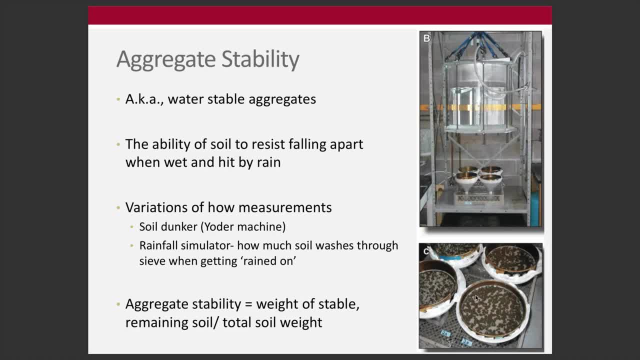 The more microbiology you have and root oxidates, the more this ability, the greater your water stable aggregates. Okay, The less tillage that you have, over time, water stable aggregates build up your porosity, your ability of that soil to exchange water and gas for the soil to. 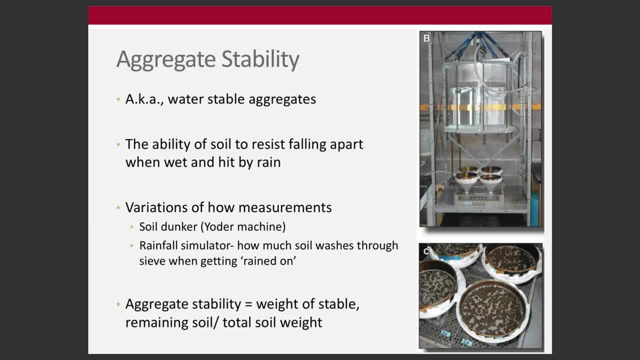 to accept water and heavy rain, Like all these things are related, Okay, And so aggregate stability can be measured a few different ways. There's a soil dunker or a yoder machine where it's moving soil through a column of water up and down and seeing how much falls apart. 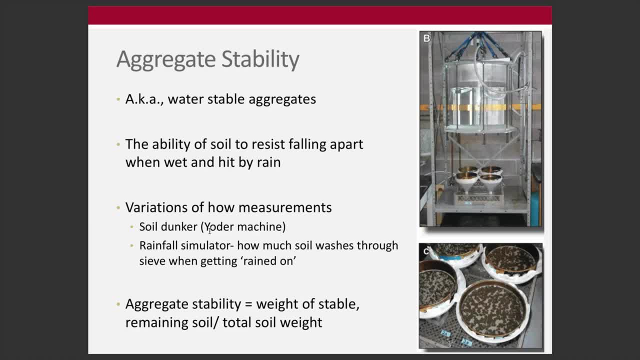 But maybe in the field or even in the lab, we can use a rainfall simulator. This is something from the Cornell manual And they've got this kind of complicated apparatus. They swing this a little bit And this is essentially. you can't see these little tiny, little micro tubes, but it's raining on the soil. 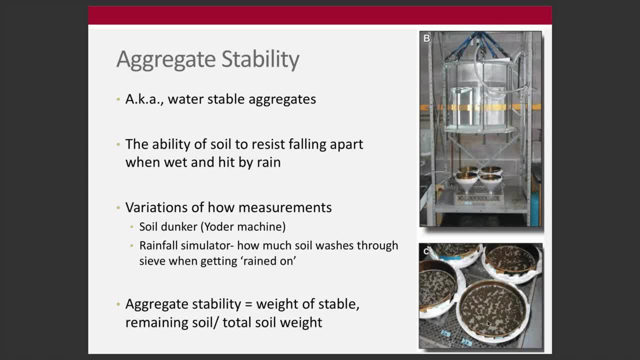 That soil either falls apart and falls through the sieve or stays together. And then that proportion that is on the sieve to begin with versus how much falls through gives you a measurement of aggregate stability. So it's essentially a percentage of the total. So this is a 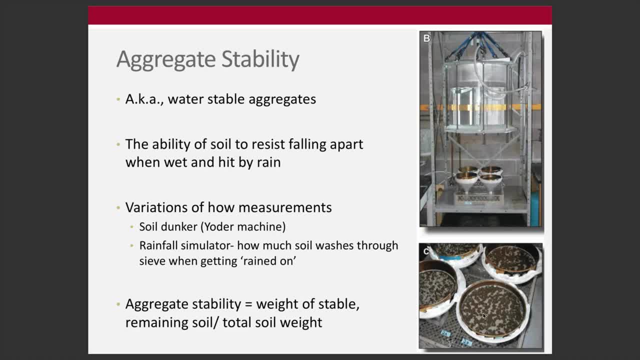 very important measurement, And Cornell has found that this is something that's a very good indicator of overall soil health. In other words, the soil has a high. you know, a lot of indicators rank very high. Aggregate stability is usually up there too. 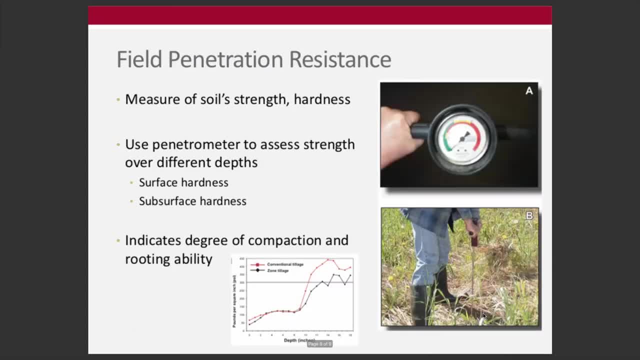 So it's a good indicator of the overall health. Field penetration resistance is done with an instrument called a penetrometer, And so this measures the soil strength or the hardness, Indicates the degree of compaction and how difficult roots are going to have in terms of getting and exploring soil space. 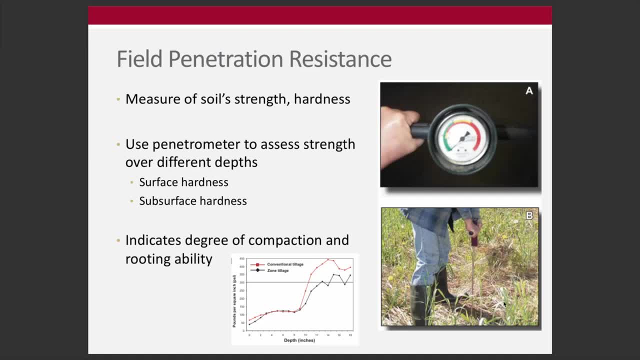 Okay, So you can do this. So this is a penetrometer. essentially It's a. it can be a little analog or digital models, Just like a metal shaft that's got a tip on it And you push that into the ground. 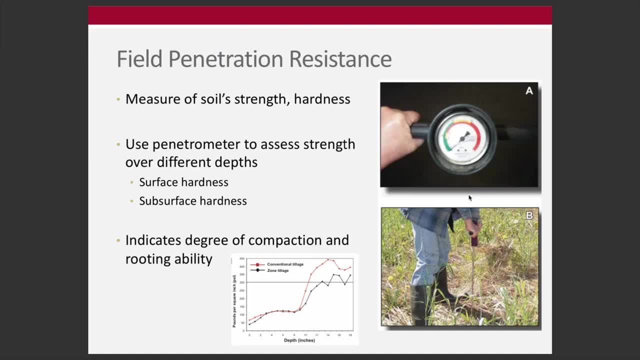 The amount of force required to push that into the ground gives you an indication of of penetrometer or penetration resistance. Okay, So you can do this at the surface. You can do this at the subsurface a number of different ways And, not surprisingly. 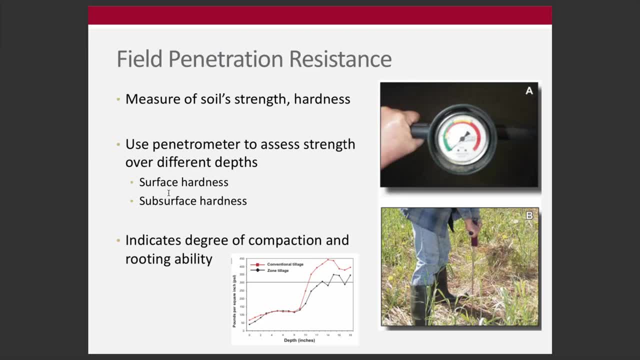 well. it's an incredibly variable measurement but it relates well to management practices, especially tillage practices, And you know again, Cornell has also found that this is an important measurement for for soil health. overall soil health, Infiltration is a very important measurement. 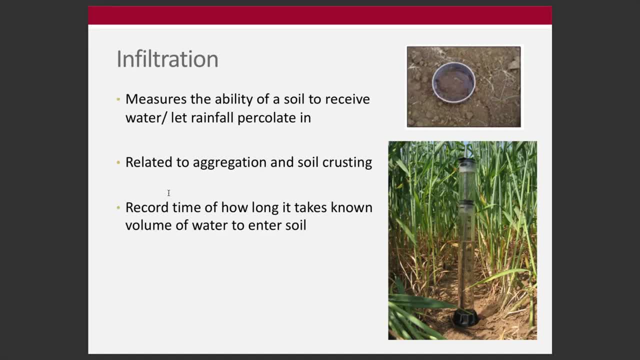 especially in the springtime, Measuring the ability of a soil to receive water or let rainfall percolate in Right? So we get these heavy rainfall events either in the spring or the summer. Is that water going to enter the soil? 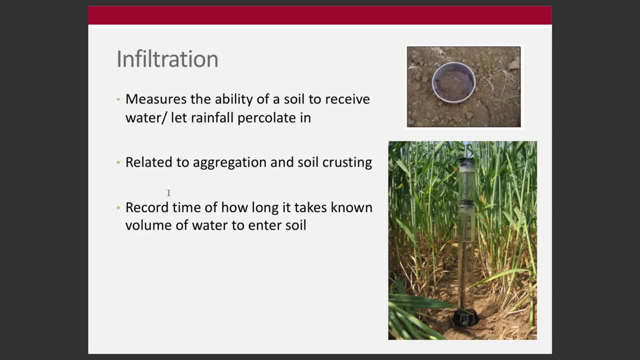 Or is it going to essentially puddle and then move via surface runoff? And when it's usually running off the surface, it's taking soil and particles with it. So that's, you know, an erosive event. The more readily a soil can accept water. 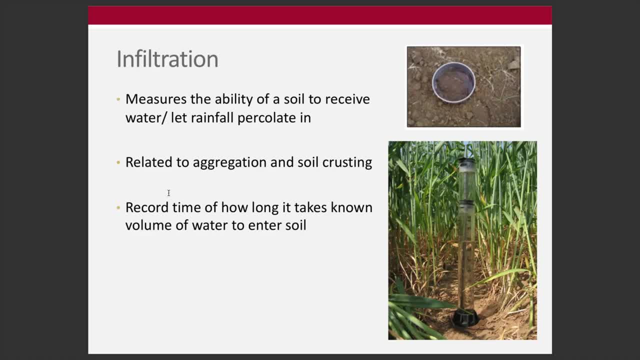 the healthier it's going to be within reason, Right? So we understand that sandy soils are going to function very differently than clay soils in this regard, So we have to scale things by soil type, You know. this is true with basically all measurements of physical structure. 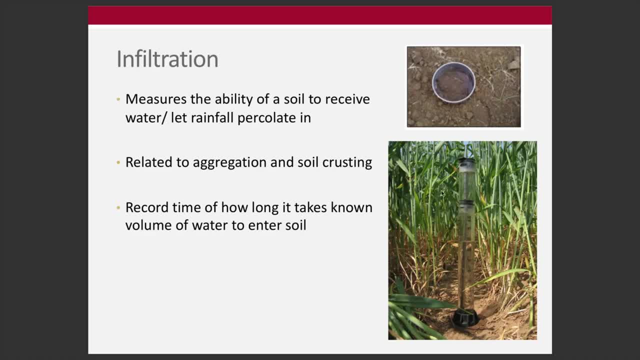 We do this commonly in our lab with these mini-disc infiltrometers, So it actually measures unsaturated hydraulic conductivity where we have a graduated cylinder here and then a a top chamber. that essentially keeps this headspace equilibrated. 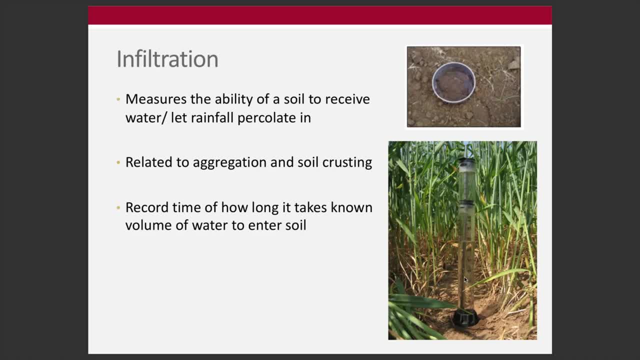 So if we pulled this thing, pulled this infiltrometer up, there would be no water that ran off. But when we make soil, the soil surface contact with that soil surface via capillary action that that water is going to get wicked into that soil. 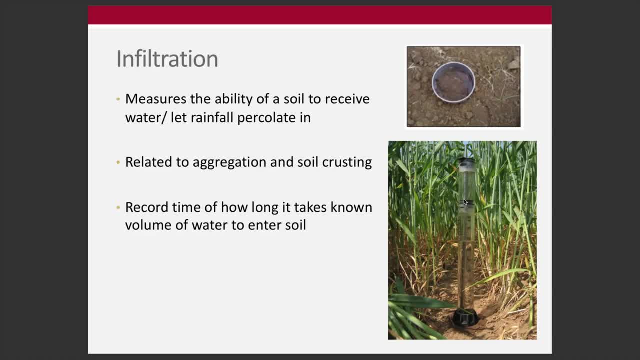 And the rate of wicking will determine essentially our infiltration rate. So some nuance with that. but essentially you know the the poor man's way of this is: just take a ring, pound it in the ground pour soil in. 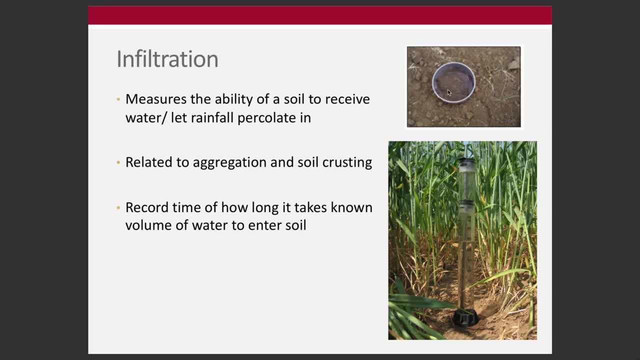 and see how, or pour water and see how long it takes for that water to to enter that soil, You know so this is. infiltration is typically a rate measurement. It's like number of inches or centimeters per minute or per hour. 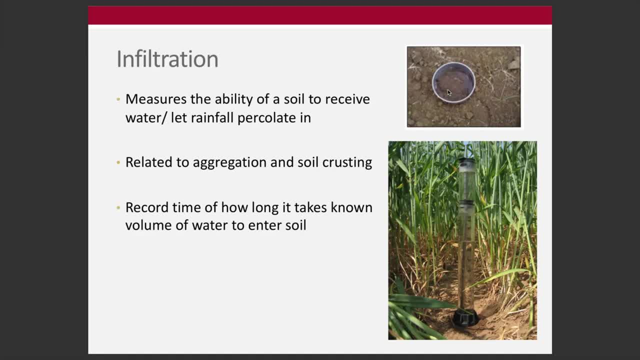 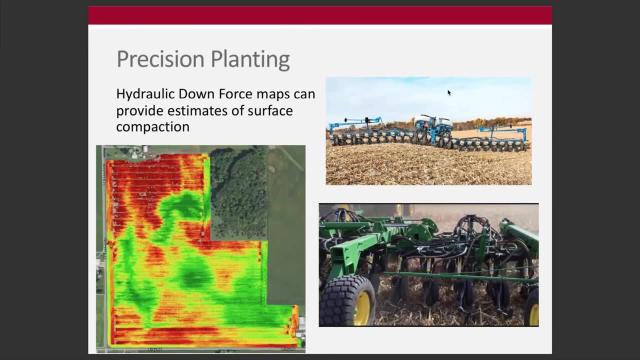 So it's like how much enters that soil on a, on a per time basis? Okay, And then so again, physical structure being a variable measurement and kind of difficult to really quantify in the field, There's other technologies that we can look at. 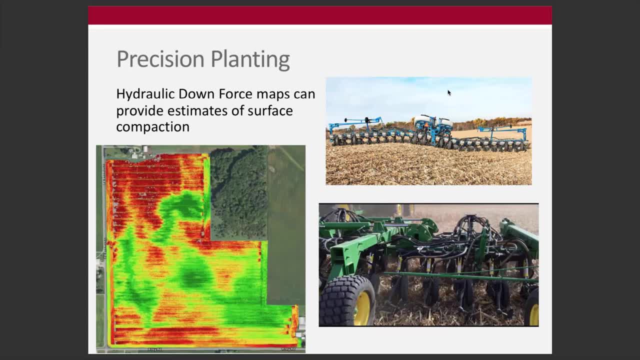 We talked in the biological indicator section about precision plantings- smart, firmer. Here's another way again from precision planning that I think we can make good strides. It's determining compaction or just surface hardness, And so precision planting makes these individual row units that apply a constant pressure on each one of these planting units. 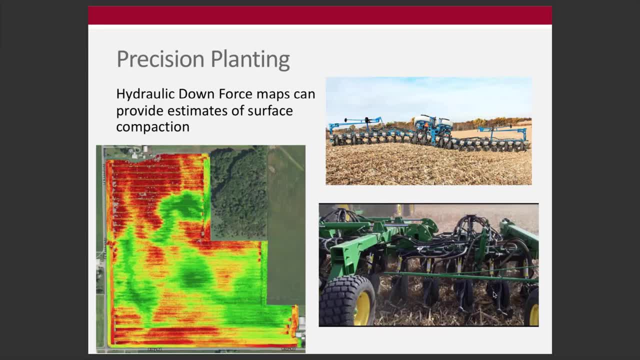 Okay, And the whole point of this is for very even seed placement. So when you're going, when you've got, say, a large planter and an uneven surface like we see right here, you know there's not, this one's not going to be placed deeper than, say, the row units up here. 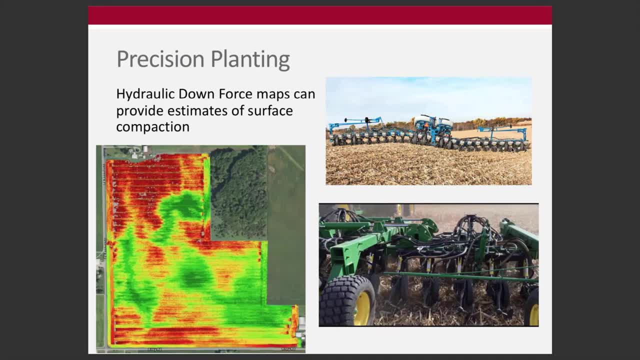 So each one of these units is supposed to be placed precisely at whatever that, whatever it's set for, like one inch, one and a half inches, two inches, That's going to mean very even emergence, And you know that's just good agronomic practice. 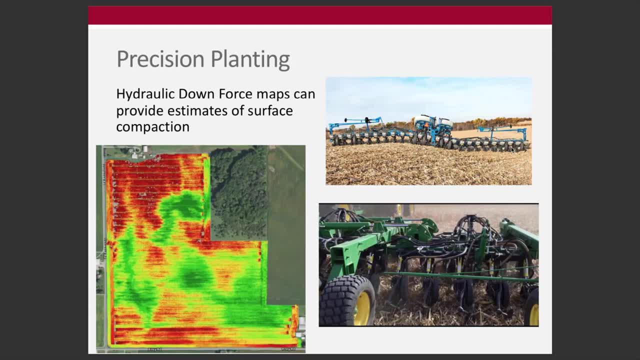 Okay, So that that has a lot of implications in terms of yield If we can get plants to emerge evenly and not compete with one another. It's keeping. these hydraulic pistons are keeping the row unit at a specific depth And sometimes it needs very little downward force to do that. 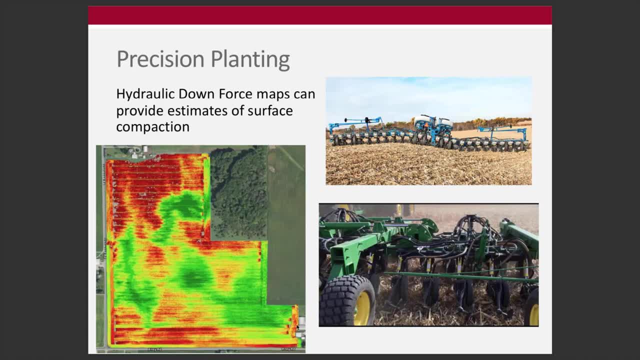 Sometimes it needs a lot. All that's recorded and logged spatially And then it prints out. you know, with their tools you can get a map here of downward force. Okay, So this is an example of how you know. 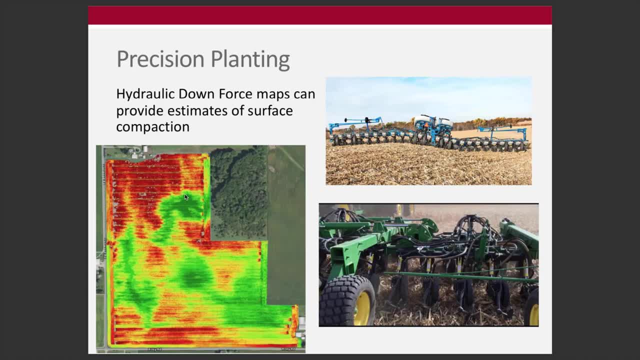 just as kind of an add on. we're going to plant anyways if we've got the capability and have these, this technology for, not maybe because we want to measure compaction, but maybe because we want to really get precise planting and get 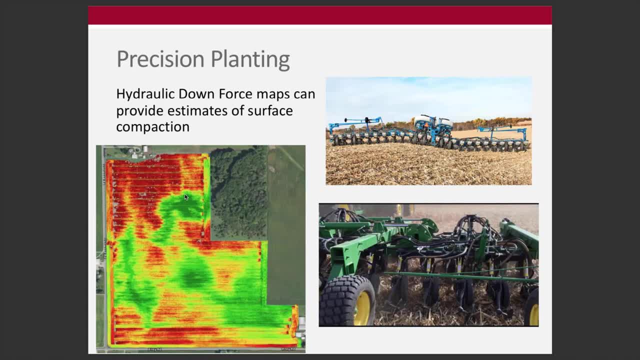 you know better, better stands that way, But we can also use that information generated from that machine as an add on for looking at surface compaction. So you know a lot of possibilities out there. but like again, how do we take?